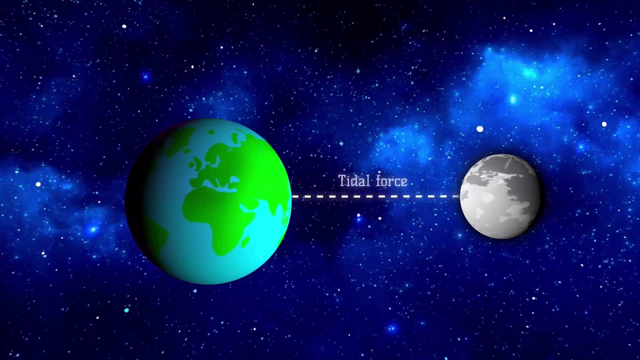 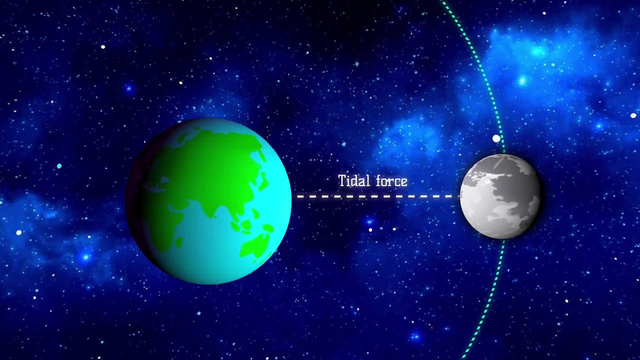 due to our earth's gravity. There is a tidal force between the earth and the moon, and it is due to this force that it becomes tidally locked and rotates continuously. This tidal force is responsible for the formation of tides on earth. In other words, just as the 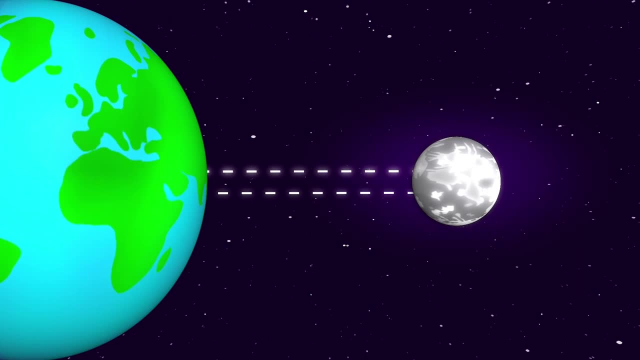 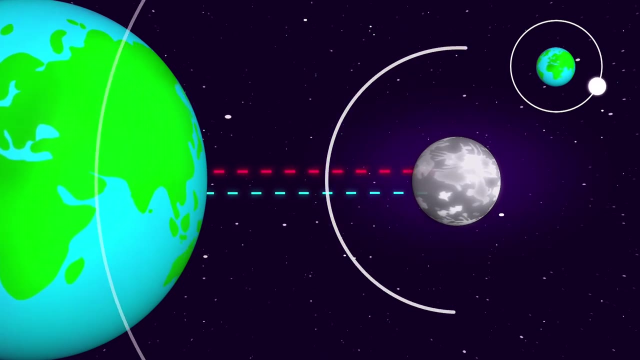 earth attracts the moon, the moon attracts the earth. Earth's gravitational pull is greater, causing the moon to orbit around. The moon's gravity is much smaller than that of the earth's, but it has little effect on the earth. That's bulging. 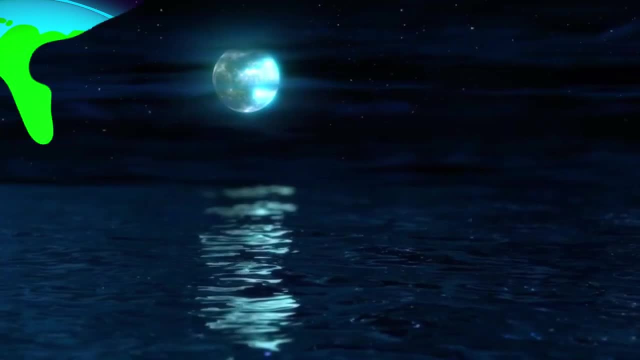 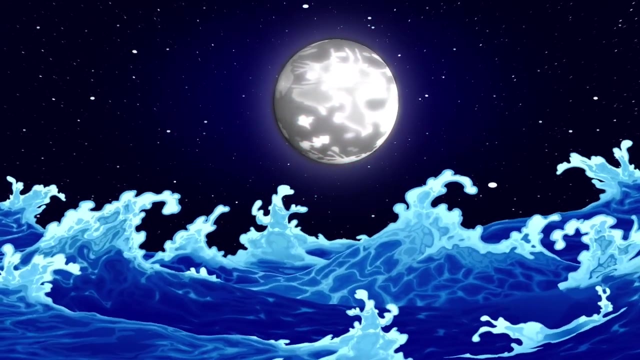 which makes the earth swell a little. Earth's surface is 70% made of water and that water is drawn to the moon. Whichever side the moon orbits around, the earth experiences the bulging effect of the moon. High tide occurs when the bulges are high and low tide occurs. 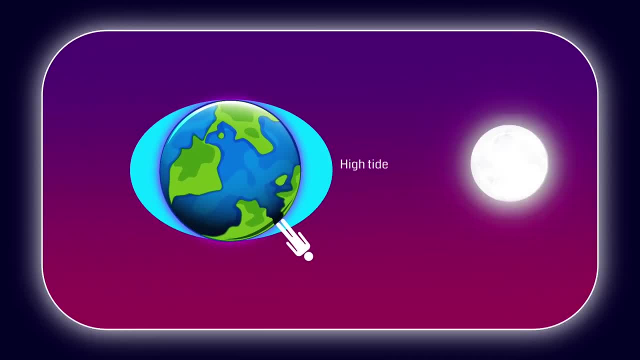 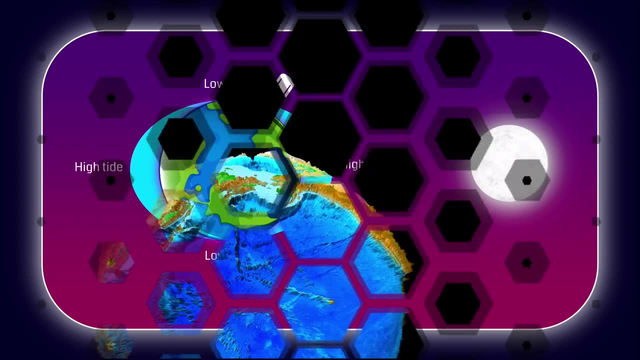 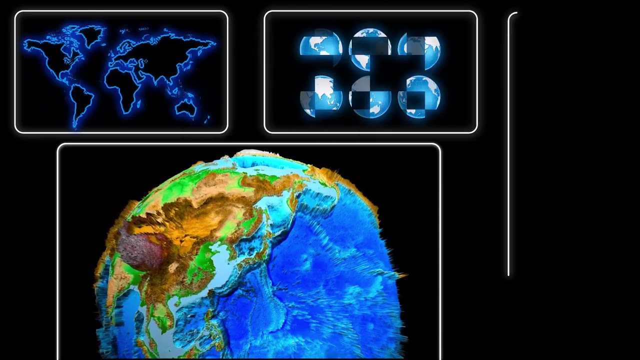 where it is low. So in 24 hours, when the earth completes one complete rotation, high tide occurs twice and low tide occurs twice. Of course, in reality, the earth isn't a small smooth ball, so tides are also affected by the presence of continents, the shape of the earth, the depth of the ocean in different locations and more. The timing and heights of the tide near you will be affected by those additional elements. We think high tide occurs only on the full moon, but the truth is that both the tides and waves are high during the full moon or the new moon. 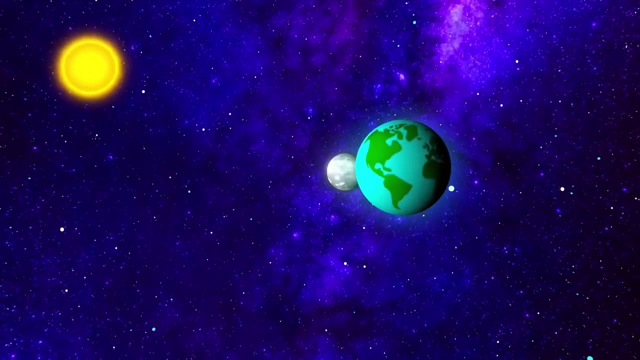 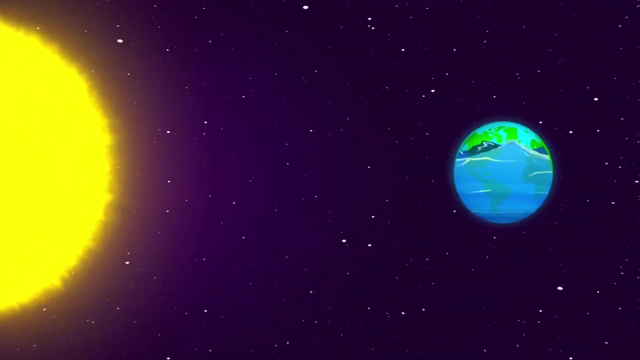 The reason for this is not only the moon, but also the sun. The main cause of these bulges on earth is usually the moon, but the sun also plays a role. The sun is the reason there are more waves and tides, especially during the full moon and new moon days, than on other days. 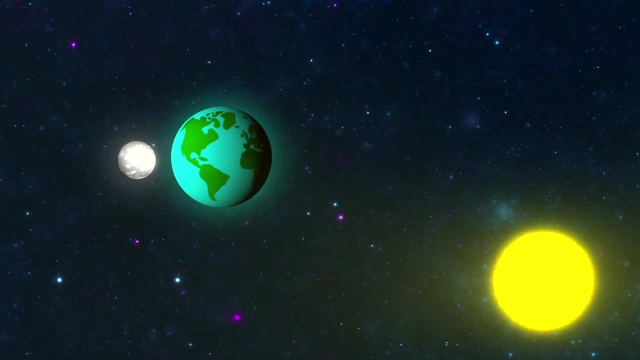 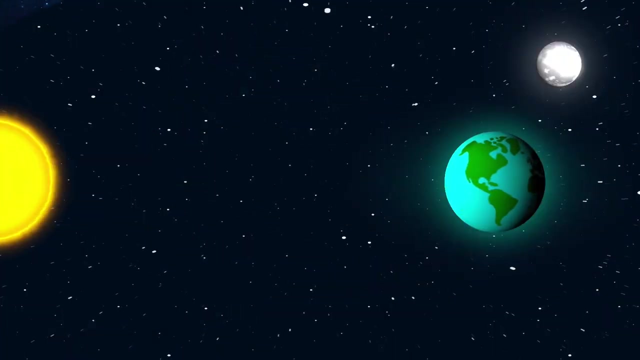 Just as the impact of the moon causes a bulge on the earth, similarly the sun, which is several thousand times more massive, also causes a bulge on the earth. On normal days, the influence of the moon is more, But what is special about full and new moon days is that the 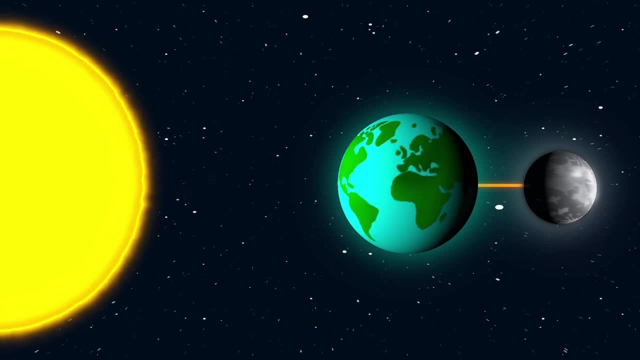 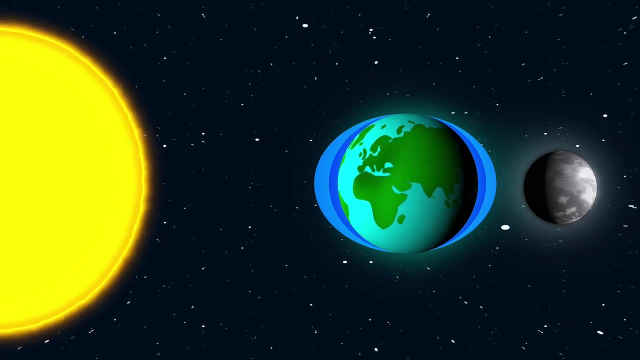 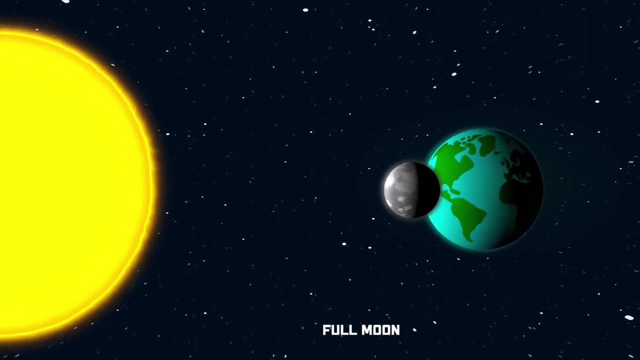 earth, sun and moon are not the same. They are the same. They are the same. They are the same. If the earth is between the sun and the moon, it is a full moon If the moon is between the sun and. 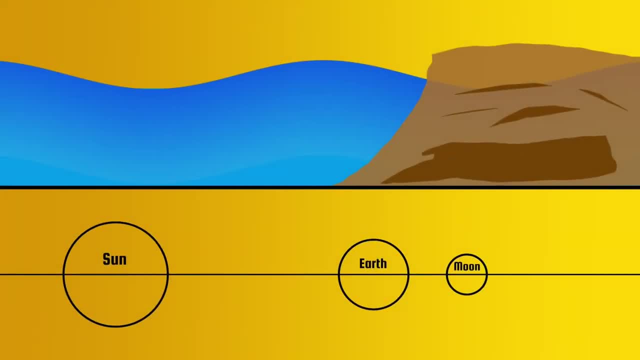 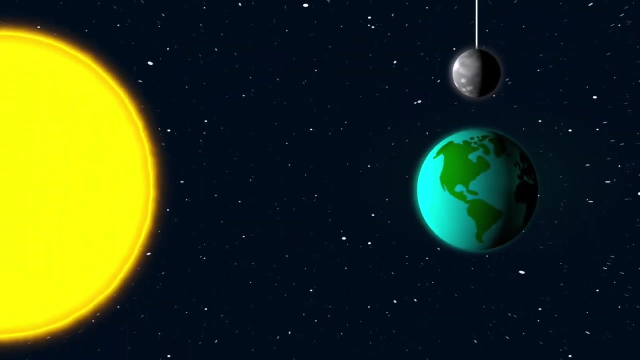 the earth. it is a new moon, Because these two are in the same straight line. during the event, there are more waves and tides. This phenomenon is called spring tides. Another phenomenon is neap tide. This means there will be few waves and tides When the moon is perpendicular to the sun and